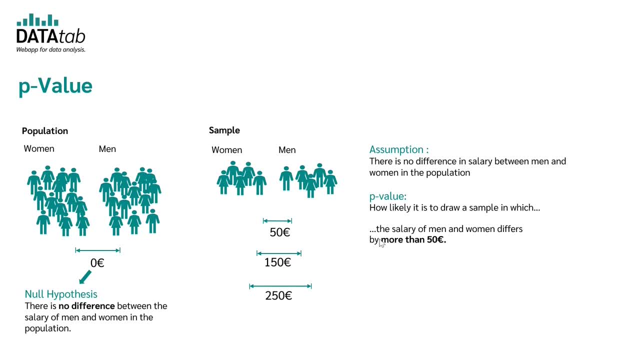 how much the salary difference is So. in the first case, the p-value tells us how much the salary difference is So in the second case, the p-value tells us how likely it is to draw a sample in which the salary of men and women differs by more than 50 euros. In the second case, the p-value would 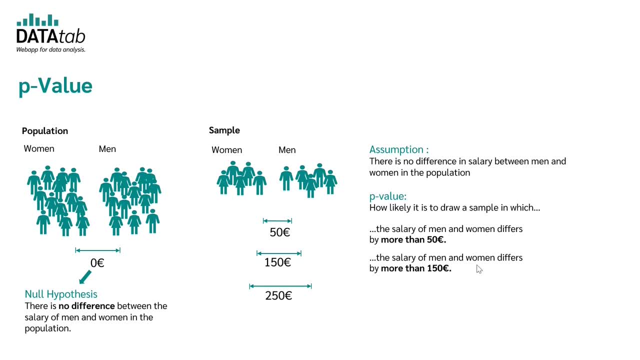 tell us how likely it is to draw a sample in which the salary difference of men and women differs by more than 150 euros. Yes, and in the third case, the p-value indicates how likely it is to draw a sample in which the salary of men and women differs by more than 150 euros. 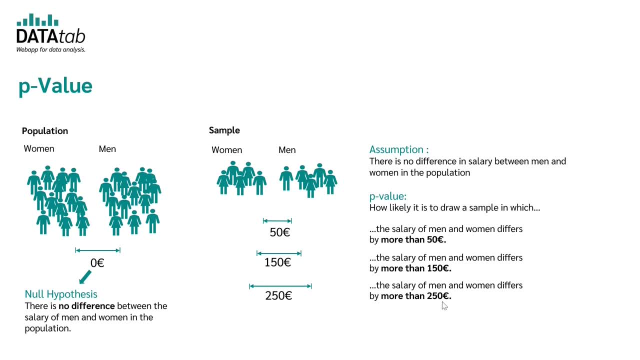 which the salary of men and women differs by more than 150 euros. Our assumption for the population still is that there is no salary difference between men and women. Okay, so what does that mean? now Let's say that you calculate the p-value for a salary difference of 250 euros and you get the 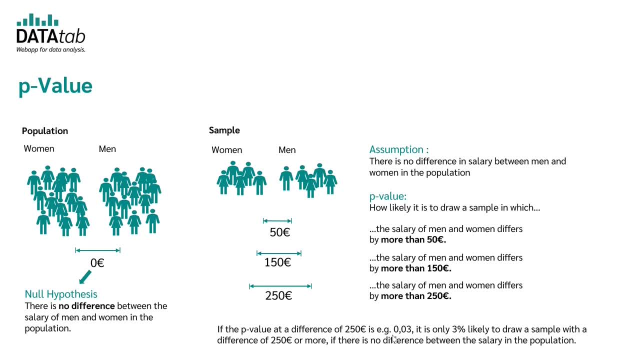 result that the p-value is, let's say, 0.03.. The fastest way to calculate the p-value is by using data tab, and I will show you how to do it in the following minutes. So what does a p-value of 0.03? 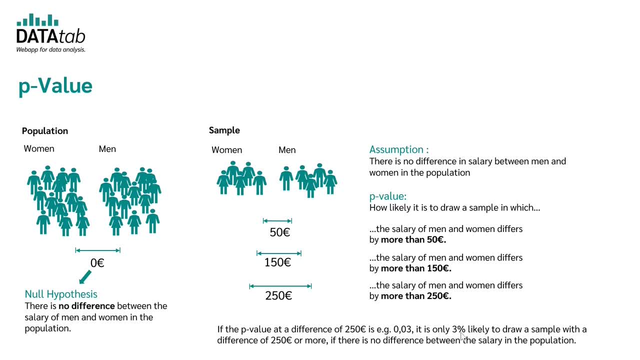 mean? The result means that it's only three percent likely to draw a sample with a salary difference of 250 euros or more, Assuming that we have no salary difference in the population. Or to say it the other way around, it is only three percent likely that this sample is drawn. 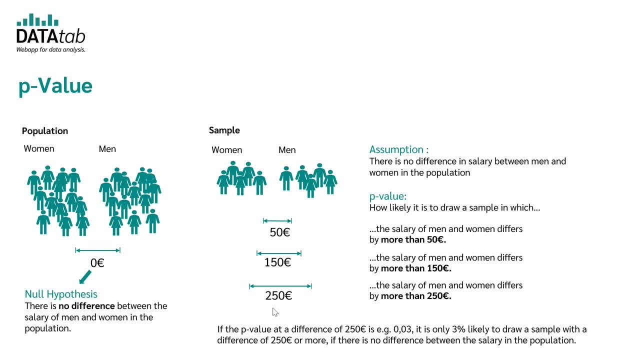 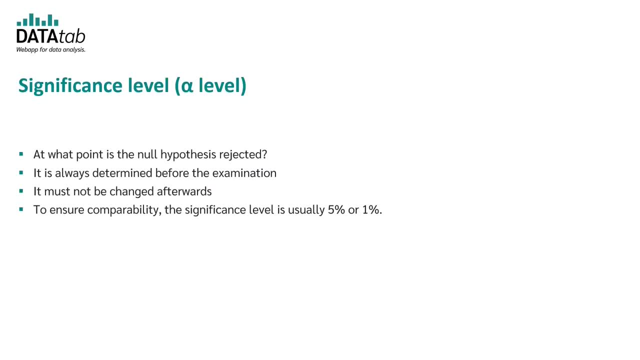 from a population. So let's say that we have a p-value of 0.03 and we have a salary difference where the null hypothesis is true, which means that there is really no difference between men and women. Okay, so now the question is: at what point can we reject the null hypothesis In order to 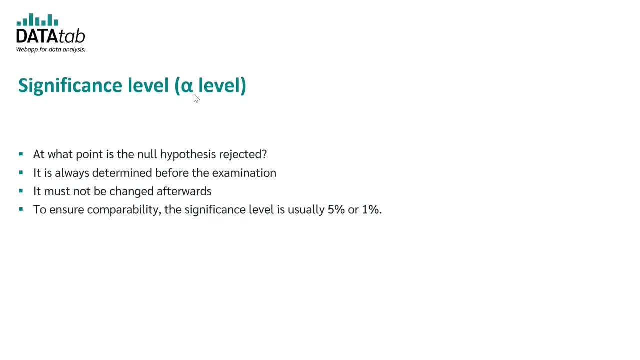 answer this question, we need to look at the alpha level, also called significance level. The significance level is always determined before the examination and it must not be changed afterwards, for example in order to get the null hypothesis. So let's say that we have a p-value of 0.03 and 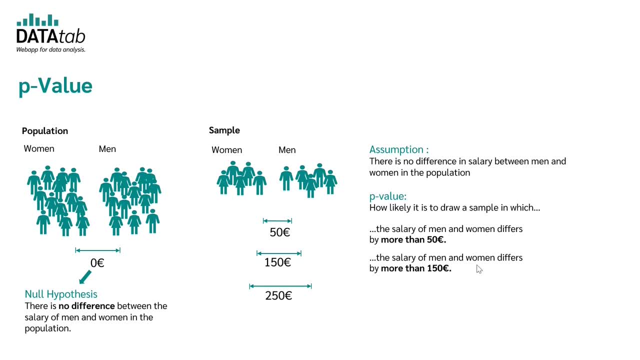 tell us how likely it is to draw a sample in which the salary difference of men and women differs by more than 150 euros. Yes, and in the third case, the p-value indicates how likely it is to draw a sample in which the salary of men and women differs by more than 150 euros. 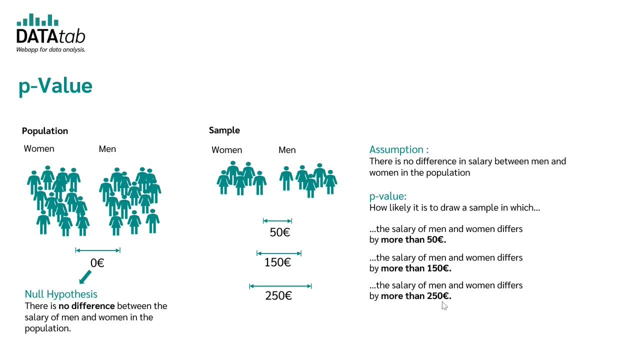 more than 250 euros. Our assumption for the population still is that there is no salary difference between men and women. Okay, so what does that mean? now Let's say that you calculate the p-value for a salary difference of 250 euros and you get the result that the p-value is. let's 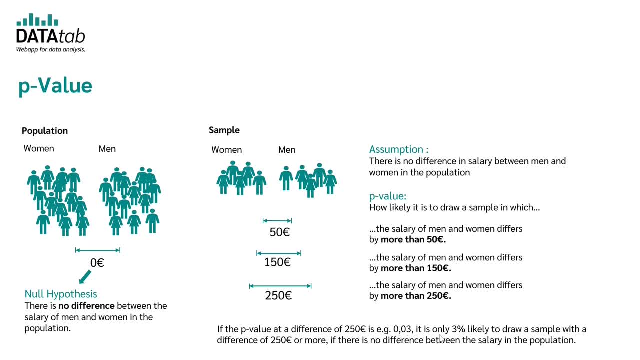 say 0.03.. The fastest way to calculate the p-value is by using data tab, and I will show you how to do it in the following minutes. So what does a p-value of 0.03 mean? The result means that it's only 3%. 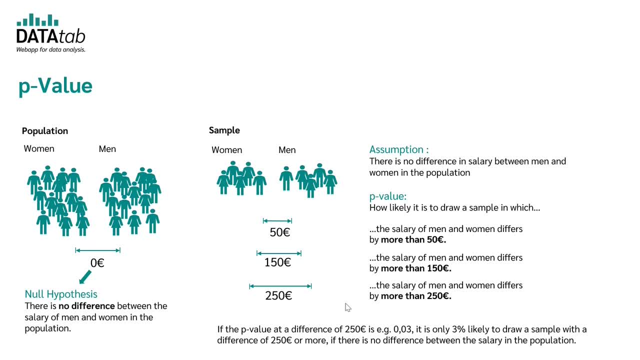 likely to draw a sample with a salary difference of 250 euros or more, Assuming that we have no salary difference in the population. Or to say it the other way around, it is only 3% likely that this sample is drawn from a population where the null hypothesis is true, which means that there is really no difference between men and 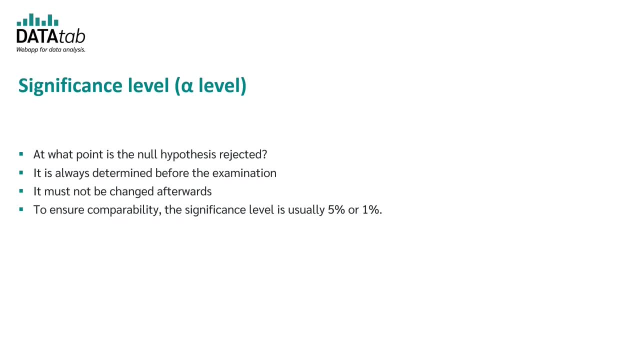 women. Okay, so now the question is: at what point can we reject the null hypothesis? In order to answer this question, we need to look at the alpha level, also called significance level. The significance level is always the same as the p-value. The p-value is always the same as the. 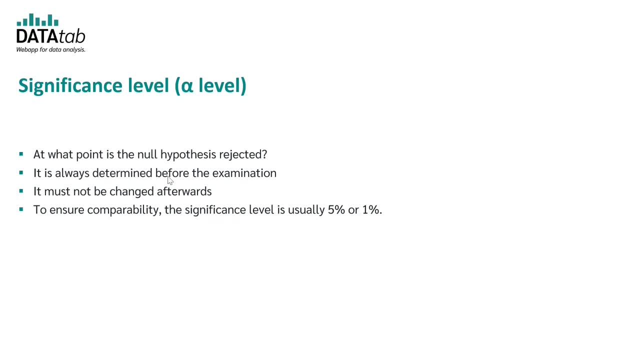 p-value. The p-value is always determined before the examination and it must not be changed afterwards, for example, in order to obtain the desired results. The significance level is usually set at 5% or it's set at 1%. This is in order to ensure a certain degree of comparability. 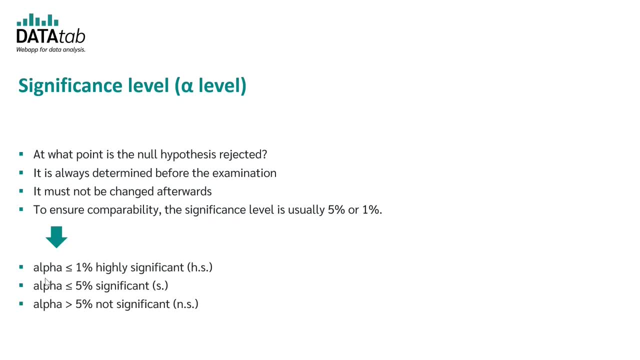 So what does it mean now? Well, an alpha level of 1% or below is called highly significant. If we have an alpha level of 5% or below, the result is called significant, and if we have an alpha level of more than 5%, the result would be not significant. Finally, we take a look at the 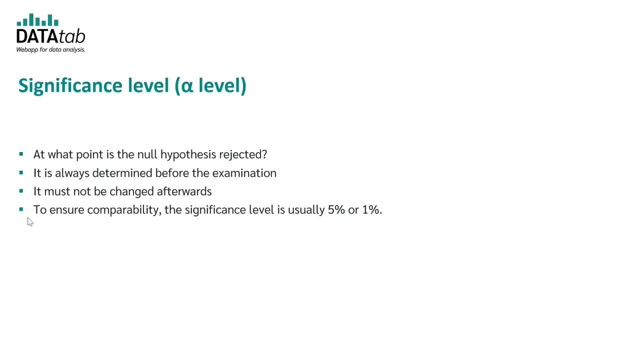 in order to obtain the desired results, The significance level is usually set at five percent, or it's set at one percent. This is in order to ensure a certain degree of comparability. So what does it mean now? Well, an alpha level of one percent or below is called highly significant. 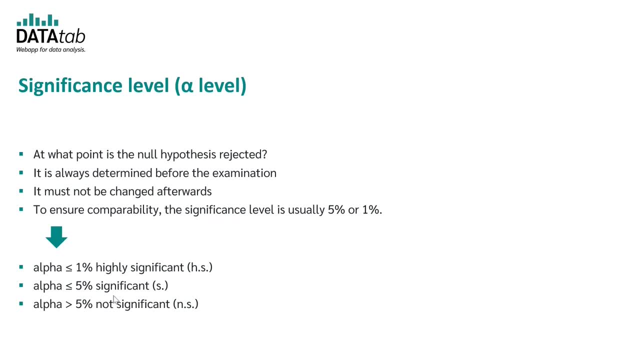 If we have an alpha level of five percent or below, the result is called significant, and if we have an alpha level of five percent or below, the result is called significant. So if we have an alpha level of more than five percent, the result would be not significant. Finally, we take a look at the 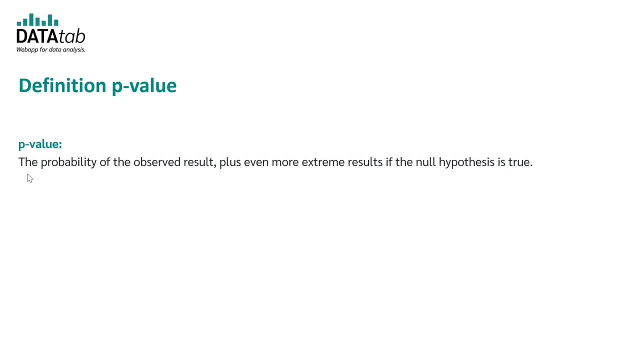 definition of the p-value. Generally, the p-value is the probability of the observed result, plus even more extreme results if the null hypothesis is true. So this might sound a bit complicated now, so let's take a look at our example again. What does it mean that the null hypothesis is true? 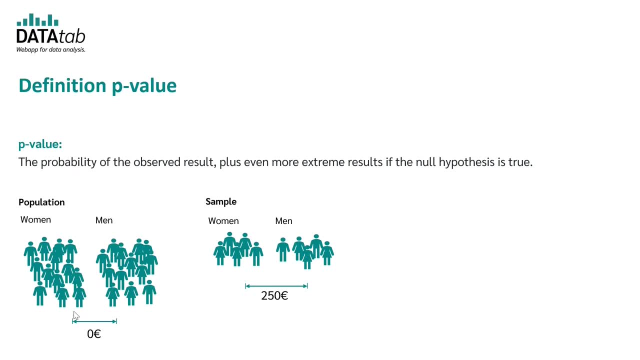 This means that we have no difference between men and women in the population regarding their salary, and the p-value now gives us the probability that we draw a sample where the salary of men and women differs by more than 250 euros, although there is no difference in the population. So let's 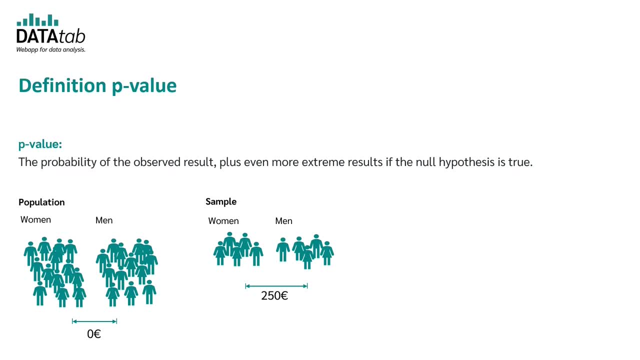 say that the p-value is 0.03.. This means that it is only three percent likely that we draw a sample where the p-value is 0.03.. So this means that we have no difference between men and women in the population regarding their salary of men and women differs by more than 250 euros if there is. 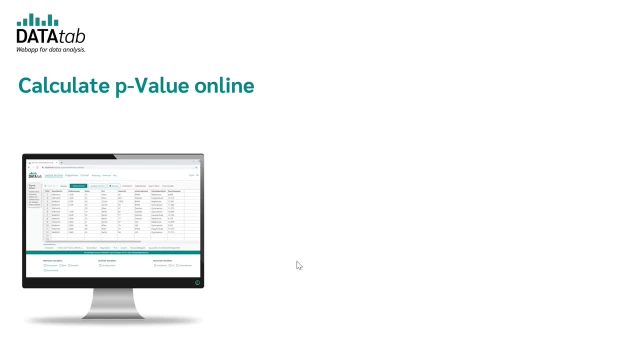 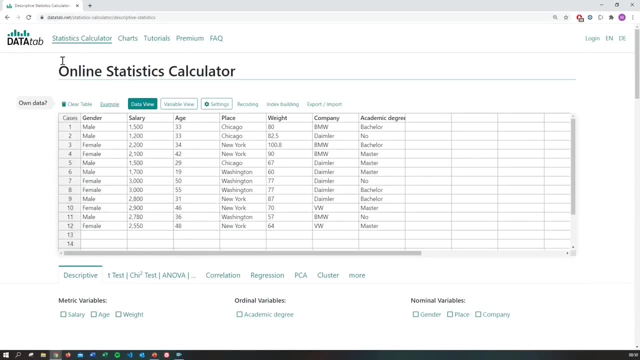 no difference in the sample. And now I'd like to show you how you can calculate the p-value with Datadab for this example. In order to do this, please visit datadabnet and go to the statistics calculator In this table. you can copy your own data now and I will use the example data. 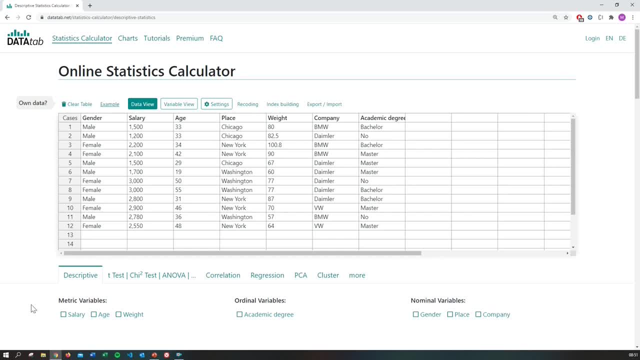 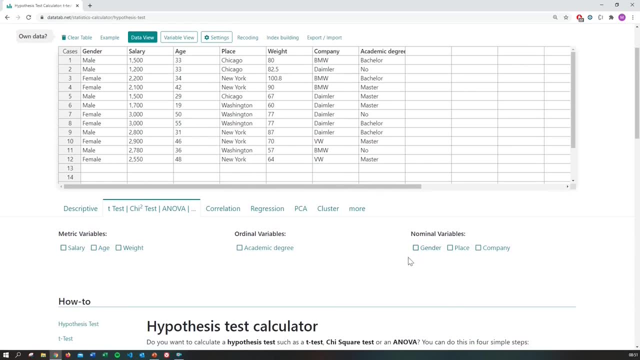 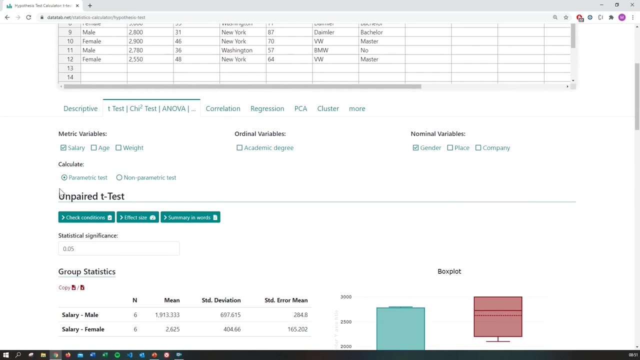 Now you can see your variables here, and then you have to open the tab t-test, and we want to analyze if the variable gender has an influence on the salary, and so we simply click on gender and salary, And now Datadab will automatically calculate a t-test for independent samples. 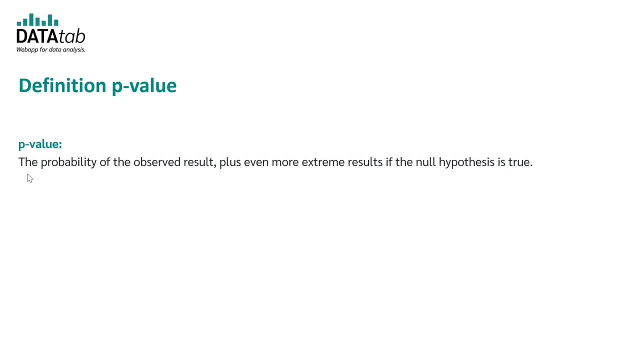 definition of the p-value. Generally, the p-value is the probability of the observed result, plus even more extreme results if the null hypothesis is true. So this might sound a bit complicated, so let's take a look at our example again. What does it mean that the null hypothesis is true? 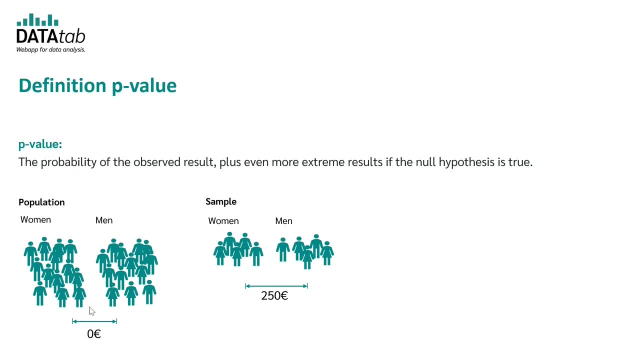 This means that we have no difference between men and women in the population regarding their salary, And the p-value now gives us the probability that we draw a sample where the salary of men and women differs by more than 250 euros, although there is no difference in the population. So let's say: 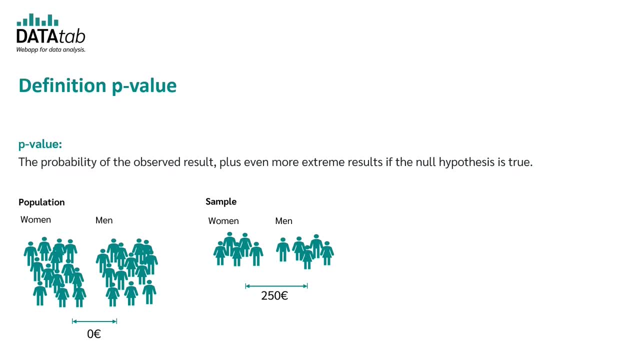 that the p-value is 0.5% and the p-value is 0.5% and the p-value is 0.5% and the p-value is 0.5%. This means that it is only 3% likely that we draw a sample where the salary of men and women 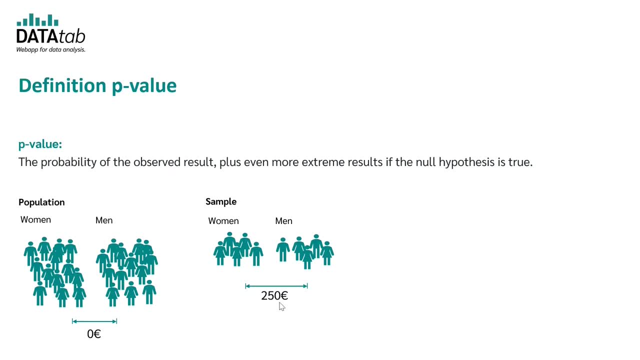 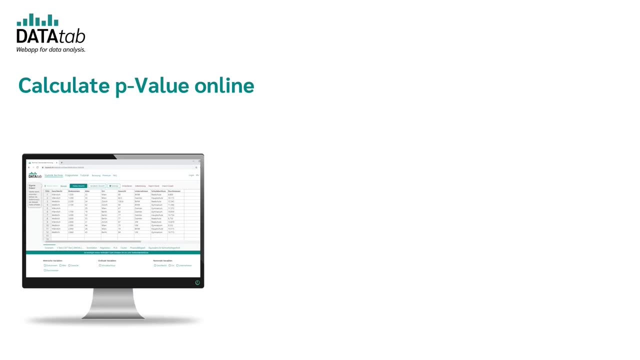 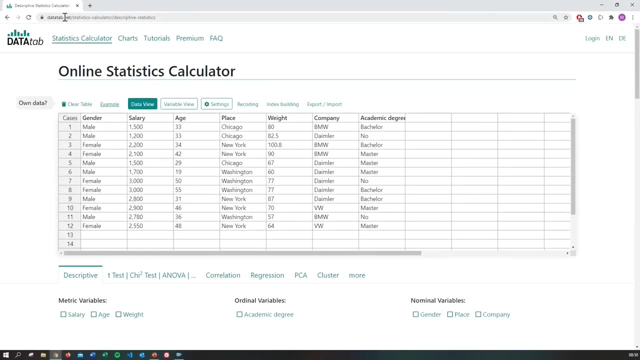 differs by more than 250 euros if there is no difference in the sample. And now I'd like to show you how you can calculate the p-value with Datadab for this example. In order to do this, please visit datadabnet and go to the statistics calculator. 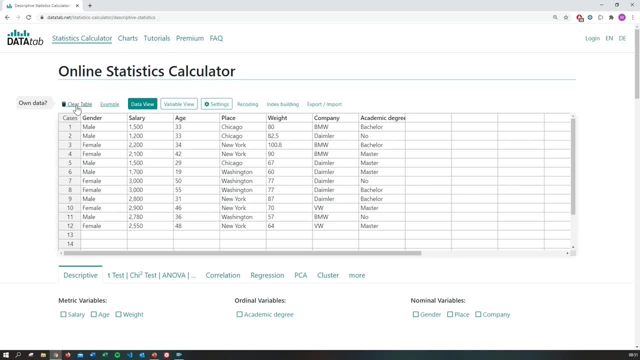 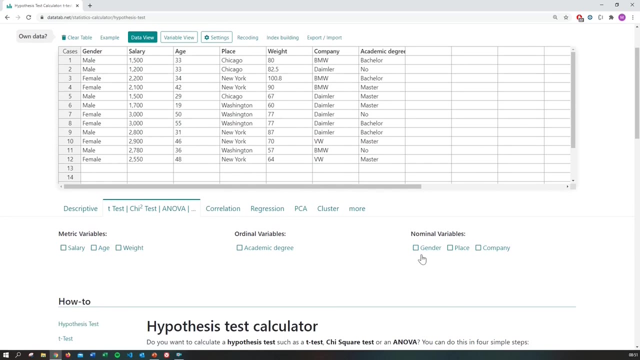 In this table. you can copy your own data now and I will use the example data Now. you can see your variables here, and then you have to open the tab t-test and we want to analyze if the variable gender has an influence on the salary, and so we simply click on gender. 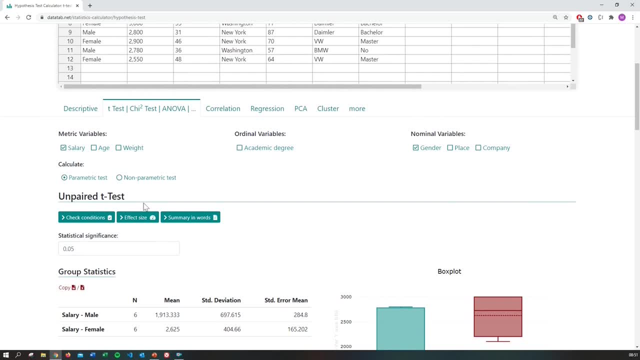 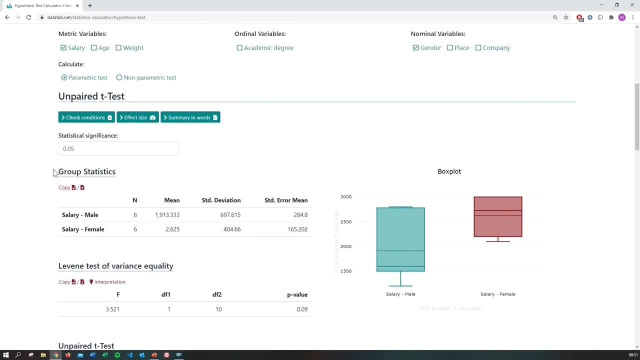 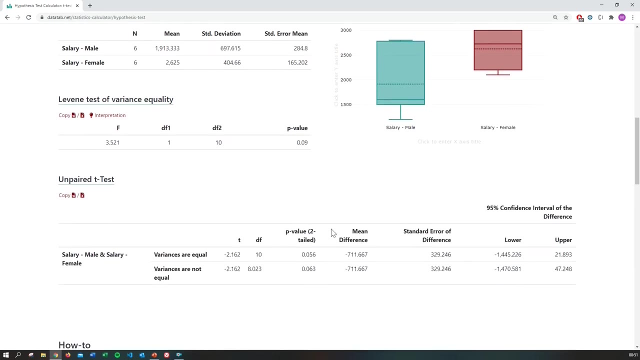 and salary. And now Datadab will automatically calculate a t-test for independent samples And in this table you can see the descriptive statistics and further below you will find the resulting p-value. If you like, you can simply click on summary in words and Datadab will give. 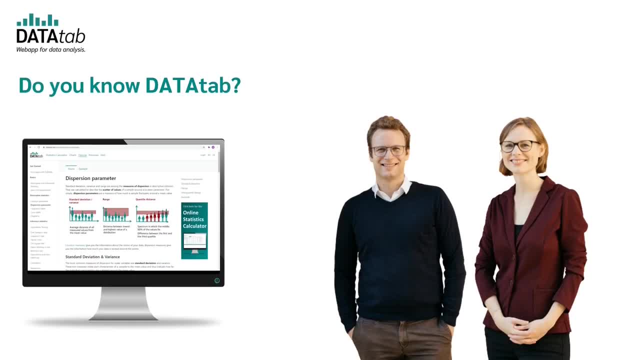 you the interpretation of your results. Okay, now you know everything about p-value and how you can easily calculate it online with Datadab. If you don't know Datadab yet, just visit datadabnet. There you will find great and helpful tutorials and you can easily analyze your data directly. 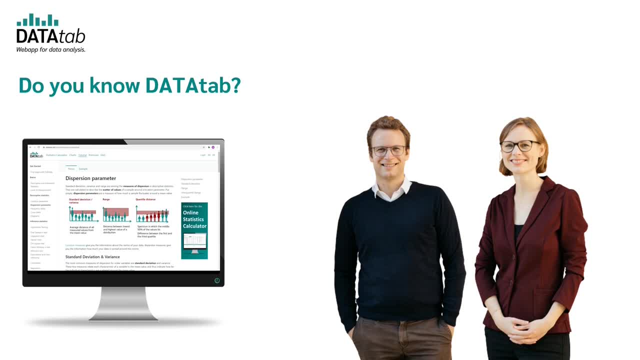 online. If you want to be informed about new videos, just subscribe this channel. Thanks for watching. 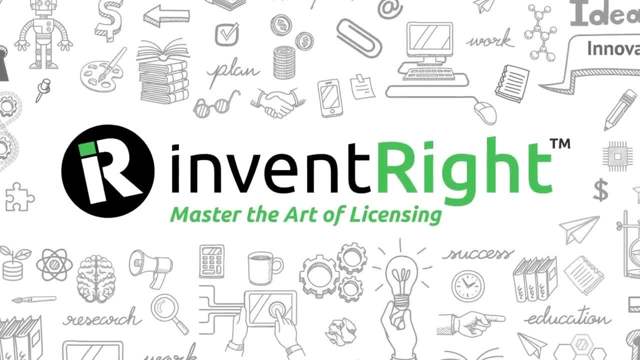 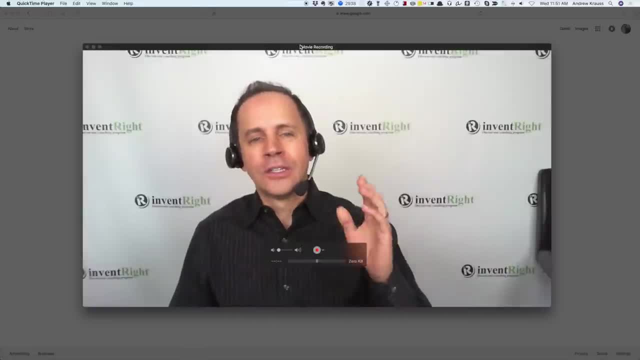 Hello and welcome to the inventrightcom show. My name is Andrew Krause. I'm the co-founder. Today, what we're going to do is give you confidence. For those of you that have never contacted a company, we're going to give you the confidence to go actually contact a few. 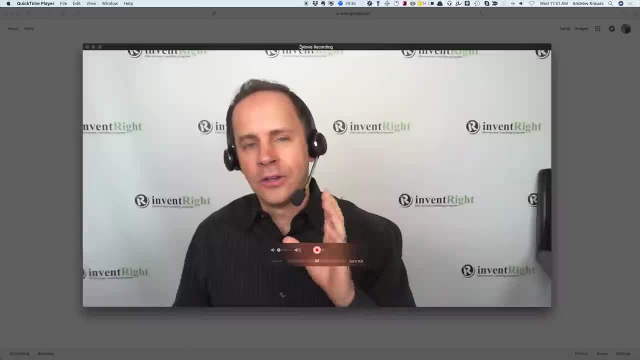 You don't have to have an idea, You don't have to contact companies for your idea. You're going to use the approach that I'm going to show you right here And it's kind of homework And I want you guys to reply in the comments down below as to how it went, And I'm going to 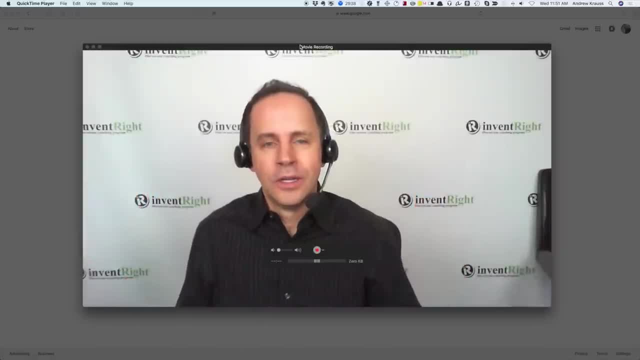 go ahead and monitor this, not forever, not for the next 10 years, but for the next couple weeks. I'm going to go ahead and monitor the comments. I want to see how you guys did So. a lot of people are really afraid of contacting companies And by doing what I'm going to show you here, 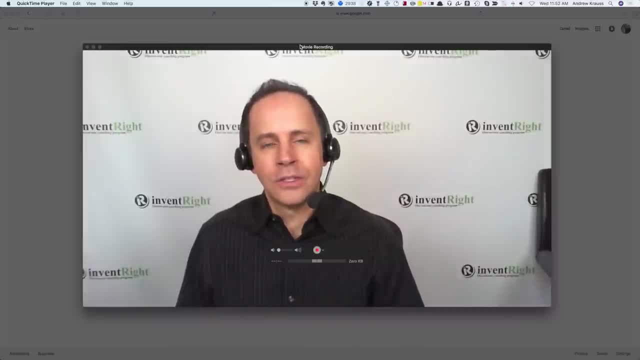 it's going to take that fear away when you realize that you can contact companies and you can submit ideas. So I'm going to show you how to just get a phone number for a couple companies and call them and ask them if you can submit an idea And just having done it. So if they say no, that's fine. 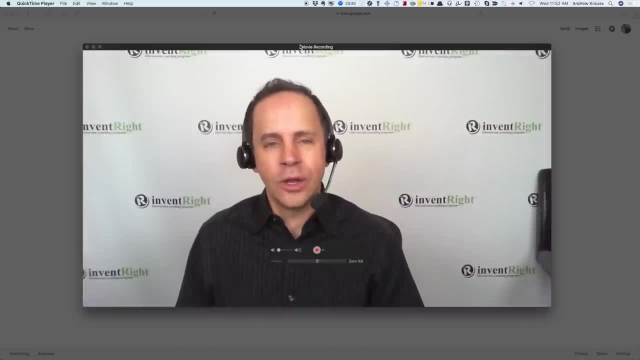 If they say yes, but I don't know what to put you with, whatever, Just that you know that you contacted a company and you took away some of that fear that you actually did it. You called a company, It wasn't scary, It was doable.